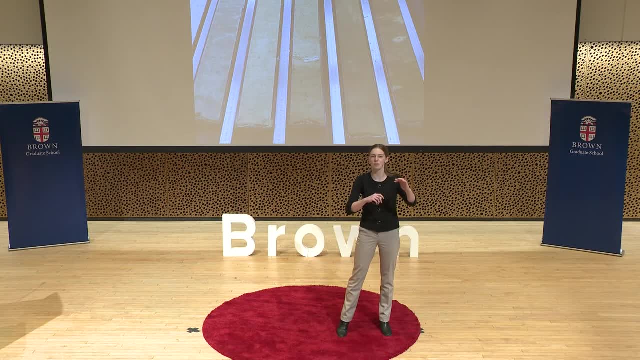 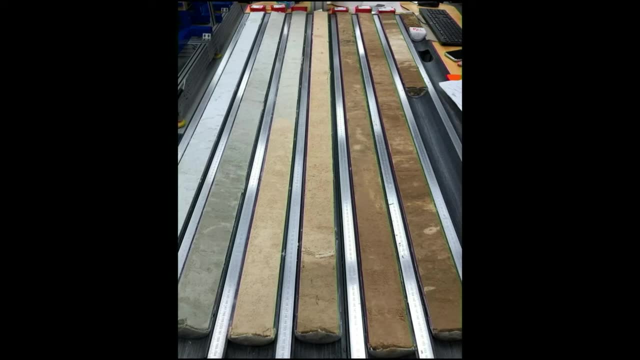 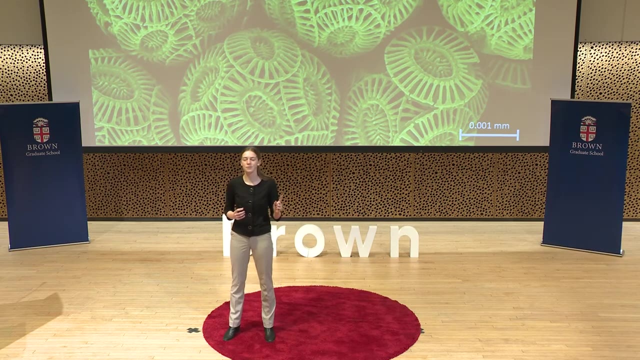 Because sediment is continuously deposited layer by layer on the ocean floor, I can construct a timeline with clues about Earth's ancient climate Within the sediment core. I am on the lookout for organic molecules and fossilized skeletons that can tell me this story about the past. 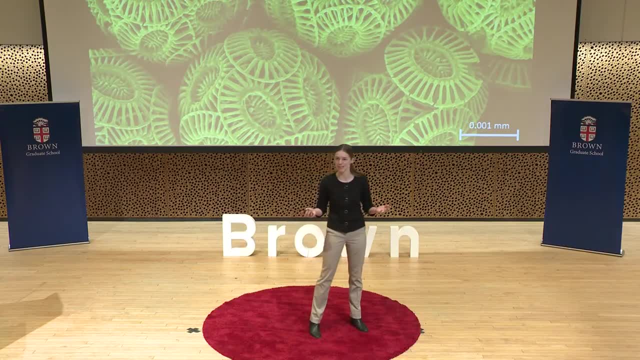 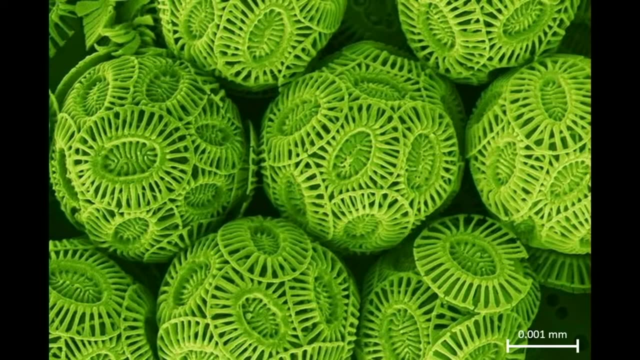 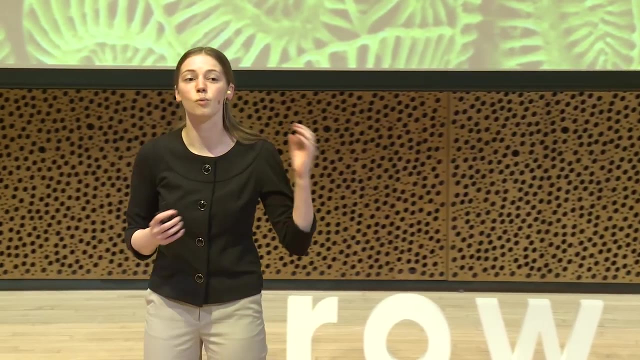 These skeletons are the ones that are most important to me. These skeletons and molecules are produced by phytoplankton, so single-celled organisms that live at the ocean's surface and record the surrounding climate conditions from the time they were alive. For example, one phytoplanktonized study produces a molecule that looks slightly different in warmer versus colder waters. 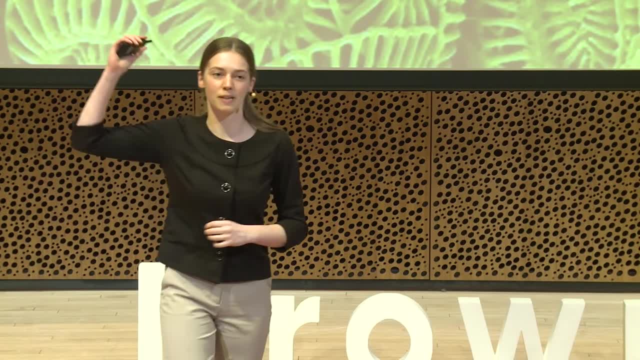 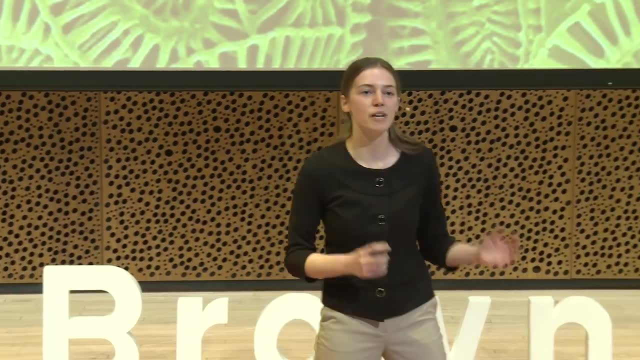 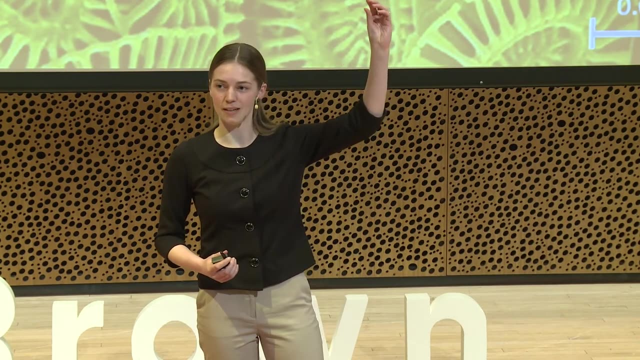 I also find a greater amount of this molecule when surface productivity is high, So I can map out past trends in productivity temperature based on the ratio and abundance of these molecules. Although living phytoplankton are found at the surface of the ocean, when they die they 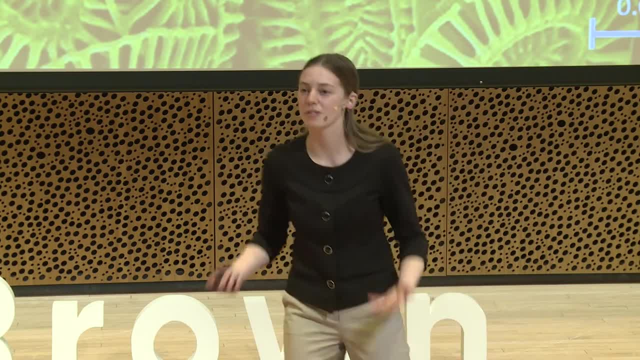 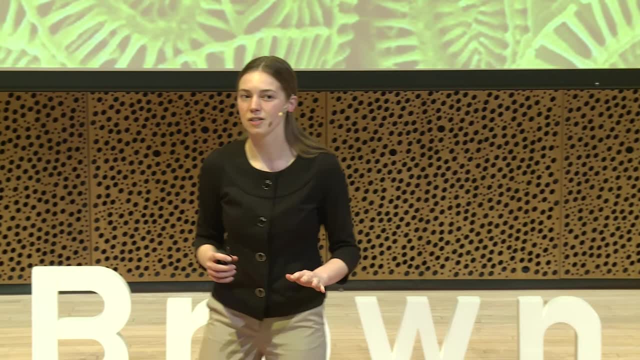 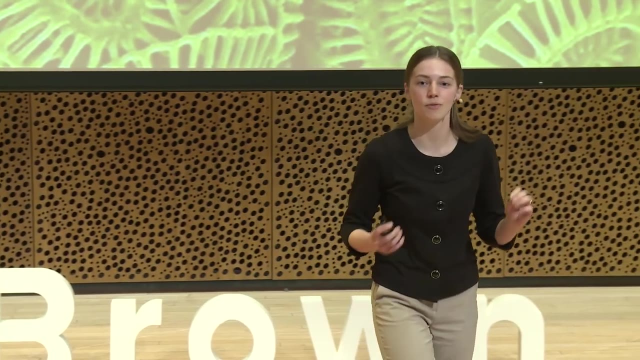 sink to the seafloor and their molecules and skeletons are preserved in the sediment that I then study. I can use these biological clues to reconstruct past temperature and productivity trends to try to evaluate whether El Nino conditions were dominant three million years ago. My research suggests that even 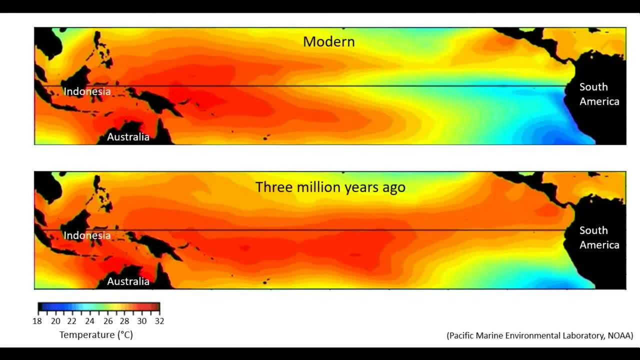 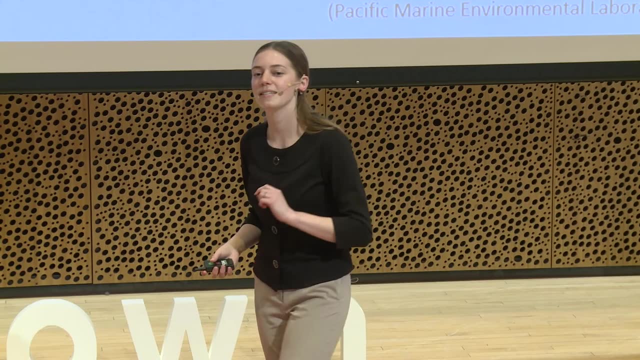 though the tropical Pacific was significantly warmer in the past, primary productivity was relatively high, and that's completely different from modern El Nino events, where warm water accompanies a crash in productivity off the coast of South America. Climate scientists still don't have a good sense. 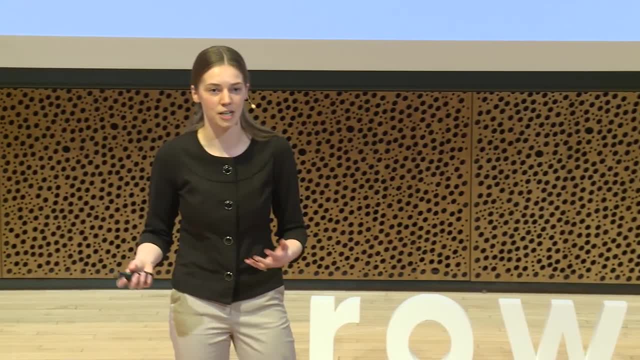 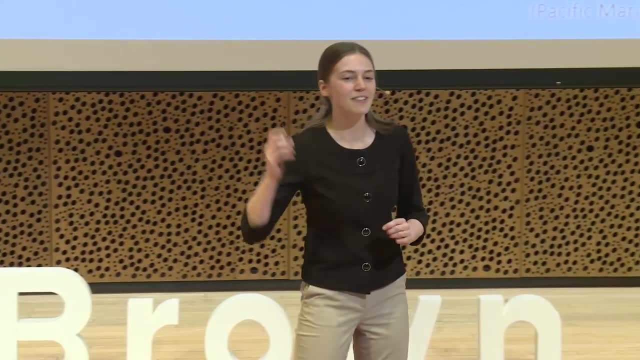 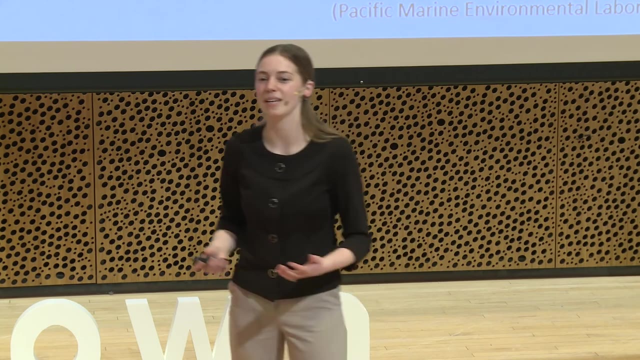 of how El Nino cycles will respond to anthropogenic changes Or human-induced global warming, But my research fills in gaps in these predictions. My results suggest that, even though droughts and flooding may become more severe in the coming decades, the productivity story is much more complex. 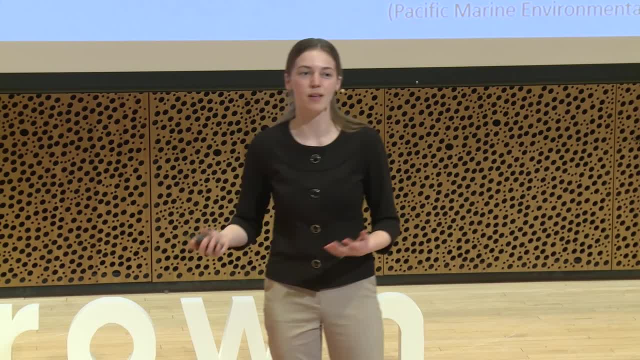 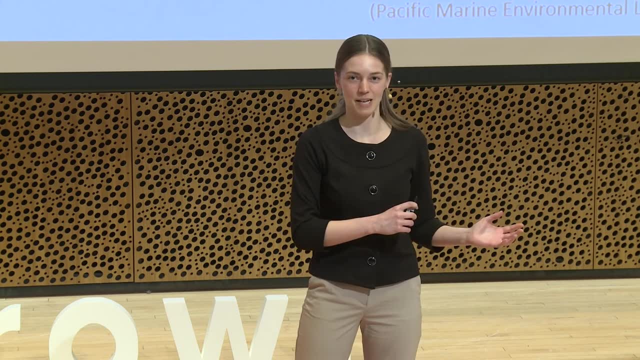 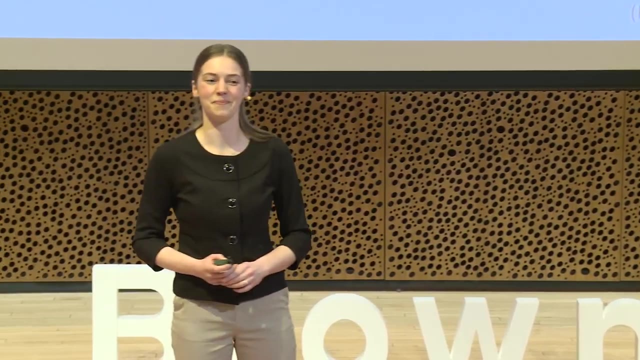 because warm water may be able to support thriving phytoplankton and fish communities. In conclusion, by reconstructing Earth's past climate, I am able to inform predictions for what Earth's climate may look like by the end of this century. Thank you,